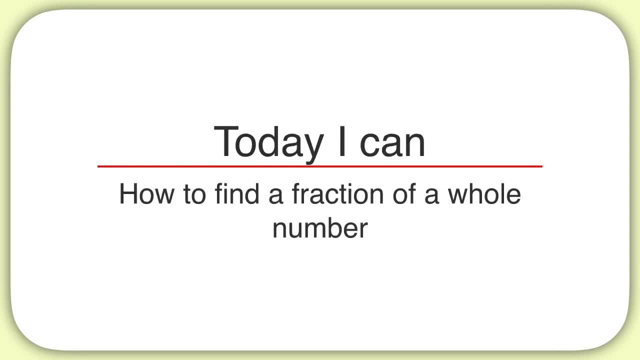 Today we are learning how to find a fraction of a whole number. First, let's find what is one fifth of ten. Well, we're looking for a piece of the number ten. so let's start by drawing this bar, and the whole thing will represent ten. Now, because we want to find 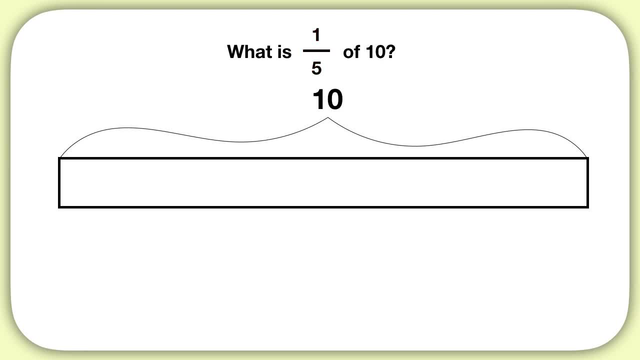 one fifth of ten. we'll take this bar and split it into five pieces, so that each piece represents one fifth of the total. But now, what should go inside each of these pieces? Well, if the entire thing is ten and we're splitting it up into one, two, three, four, 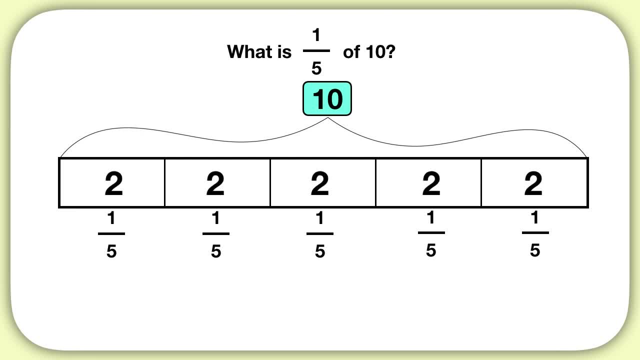 five different groups, then each group will have two in it. Now we could say that one fifth of ten is just two. Let's practice one of these together. What is one third of twelve? Let's start by drawing another one of these bar models. How much should this whole bar? 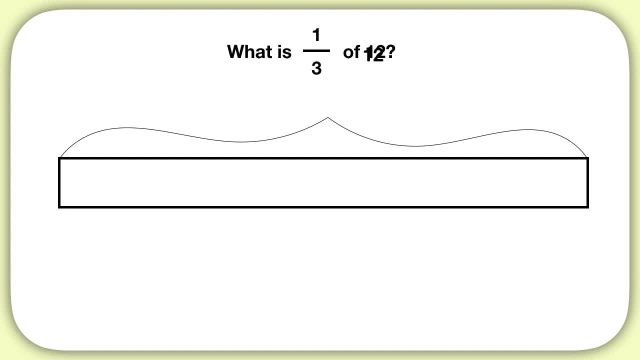 represent. This whole bar will represent twelve. Now I'm looking for one third of this. so how many pieces should I split this bar into? Because I'm looking for one third? I will split it into three pieces. Now, each piece of this bar represents one third of the total. Now, if the entire bar is twelve, how much? 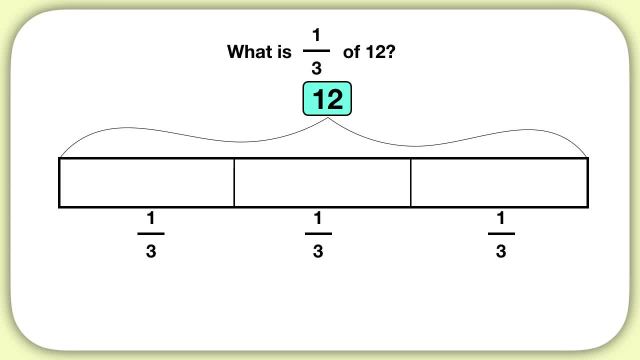 will be in each of these pieces. When we split twelve into three pieces, each piece will have four. So what is one third of twelve? zzzz, zzzz, zzzz, zzzz, zzzz, zzzz. 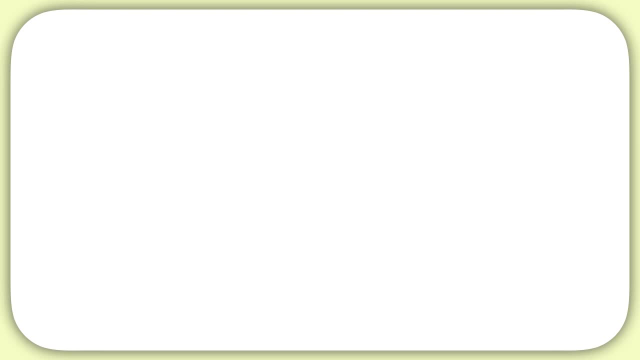 zzzz. One third of twelve, that's four. Here's another problem to practice with. Let's find what is one fourth of twenty. We'll start with our twenty and draw a bar that all together represents twenty. Now how many pieces should I split this bar into? 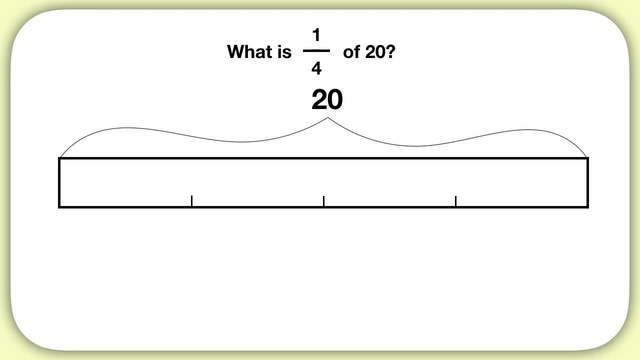 Because we're looking for one fourth, we'll split it into four sections. That way, each piece represents one fourth of the total. Now, what number should go into each piece of this bar? Well, the entire thing is twenty and it's being split into one, two, three, four sections. 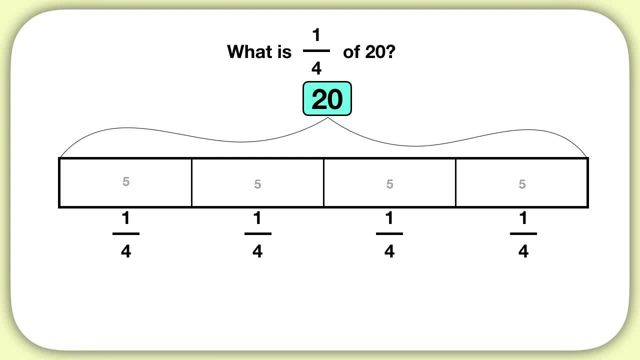 When you split twenty into four groups, each group will have five in it. So now, what is one fourth of twenty? Well, one fourth of twenty is five. Now it's time for you to practice on your own. What is one fifth of thirty?